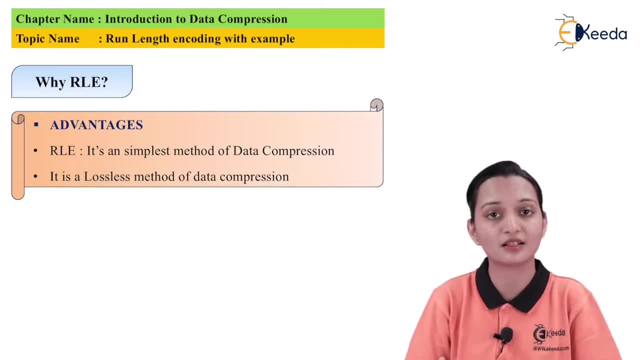 both kind of methods in our hand, like a sliding window technique, dictionary based window technique, for example LZ77, LZ78 and LZW. then also why we are going for RLA. The answer is it is advantageous in two ways. The first main advantage is it is the simplest method. 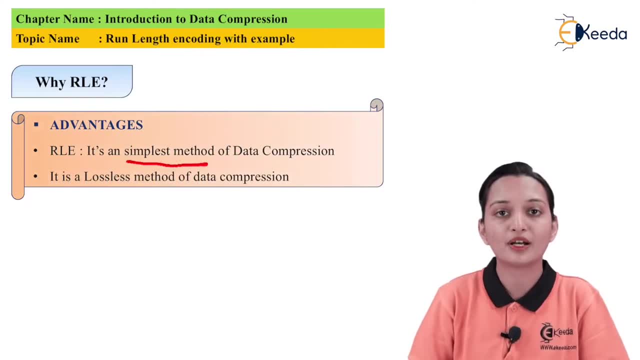 of the data compression That means for LZ77,, LZ78,, LZW and so on, Whatever time, and the steps, complicated steps. that means the drawing of table and all that. things we required comparatively in RLA we don't require to. 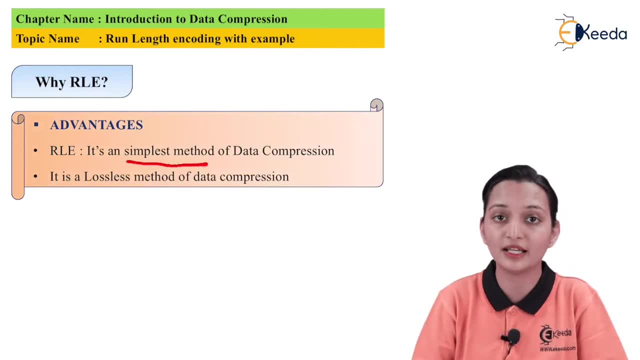 do all these things. The steps to do the RLA- encoding and decoding- are very simple as compared to the other method steps, So it is an simplest method of the data compression. This is the first main advantage advantage of this RLE. that means it requires less time to encode the data. it requires less. 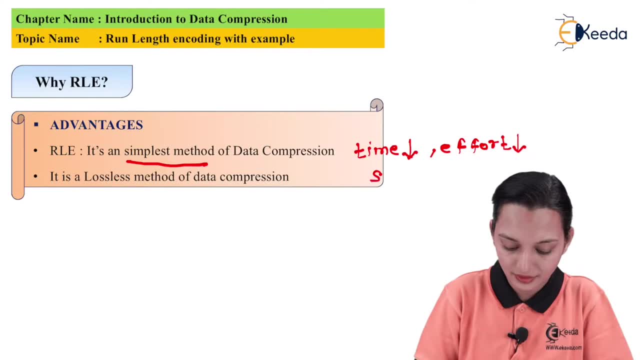 efforts and simple form. so this is the simplest method. and the second thing is: it is the lossless method of data compression. lossless and lossy: there is a difference between these two terms. in the lossless method, whatever the input we try to provide to our encoder, that complete 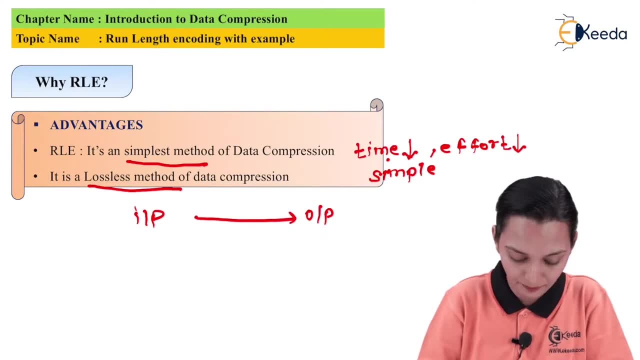 input we can achieve at the output side. so x input if I am going to provide to the input side, then after decoding that data I am again getting the x output. so there is no any loss of the data. that means no loss of the data occurs and hence always the lossless method. 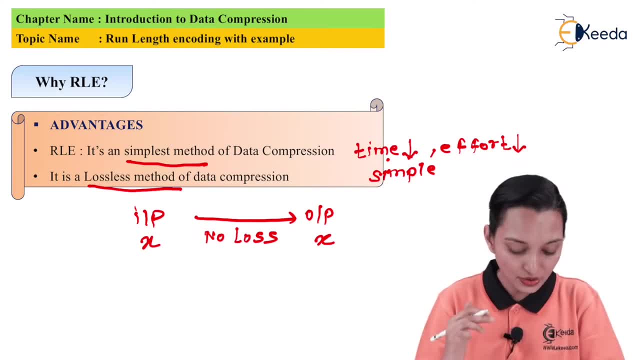 are more useful for the data compression, and so that the first thing is that it is a lossless method. so we will of course go for RLE, but not only for RLE. if we are only taking the advantage as a lossless method, then we are having what? LZW, LZ77 and all that methods in our hand, but then 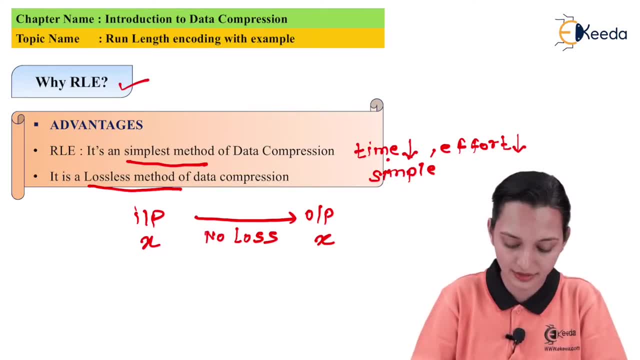 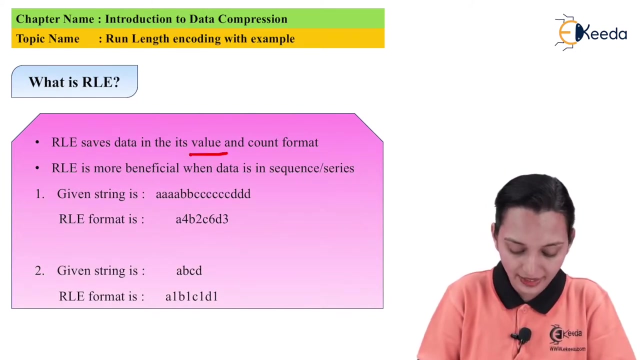 also why RLE? because it is simplest method. why simplest? because it requires less time, less effort to encode as well as to decode the data. now we will see why the name is RLE, that is, run length encoding. so what is this RLE? it saves the data in its value and count format. this 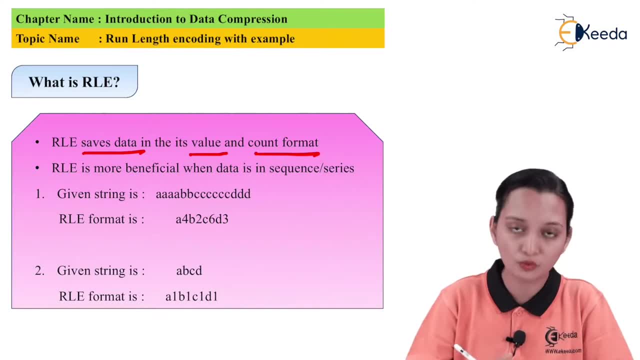 particular algorithm will try to save the data, but what kind of input it has? it has the input of sequence, of multiple sequence of data. So what is this? RLE? So sequence of multiple symbols or multiple characters are always we can found in each. 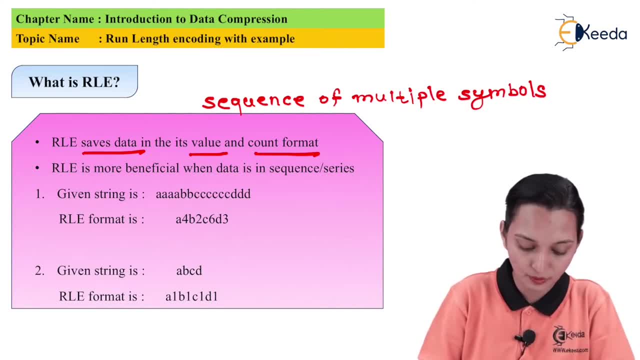 and every algorithm, but here the most probably similar sequence of multiple symbols it has in its particular string. and then we have to save the string or save the data which is in string In its value and count format, and this similar sequence of multiple symbols can be. we can. 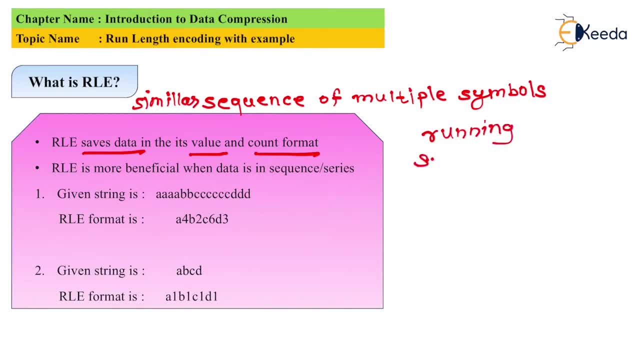 treat them as a running sequence and hence only it is known as run length encoding. that is nothing but what RLE. Now it is more beneficial when the data is in sequence or series, for example. I will first explain you few examples. For example, the given string is this: is a, a, a, a, b, b, c, c, c, c c c and d, d d. that means what? 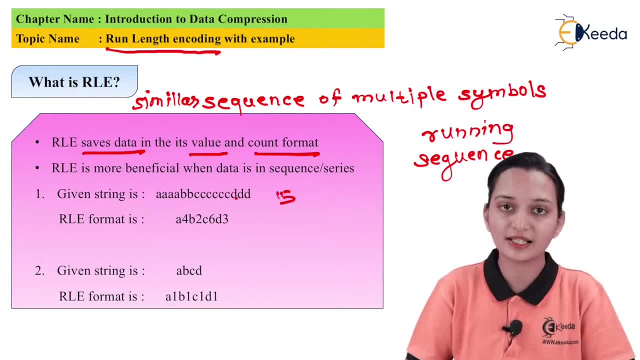 how many bits are in this particular string. that means, in the given string, 15 bits are there? 15 characters are there. and now using this run length encoding. why run length? because, see, it is a running sequence of the similar characters or symbols, but the symbols are. 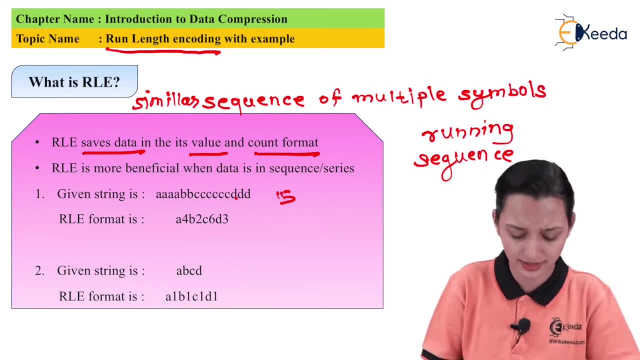 multiple also. that means a is there, b is there, c is there, as well, as d is present in the given string. now, if I want to write down its RLE format, then what I can do, write down its value and its count. so the first character is what, a. so this is nothing but value and 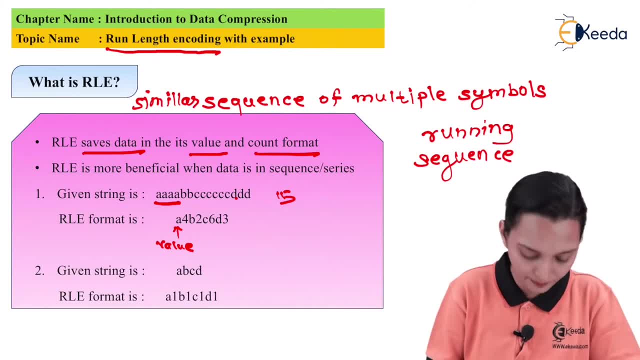 how many times a appears in your this given string: one, two, three, four, four times. so this four is nothing but what count. So it is very simple to convert any format into the RLE format now. the next thing is that the next character is what b. so b is nothing but the value, data value and how many. 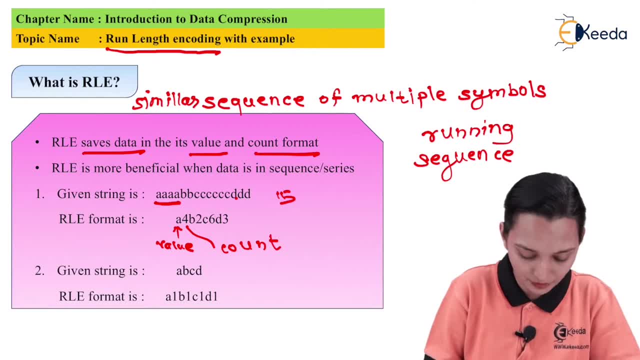 times count. it has in this string one, two, so two will be the count. next one is c. so c is nothing but what value of the data? How many times? c repeats six times, so c6 is nothing but the compressed form of the data in the RLE. 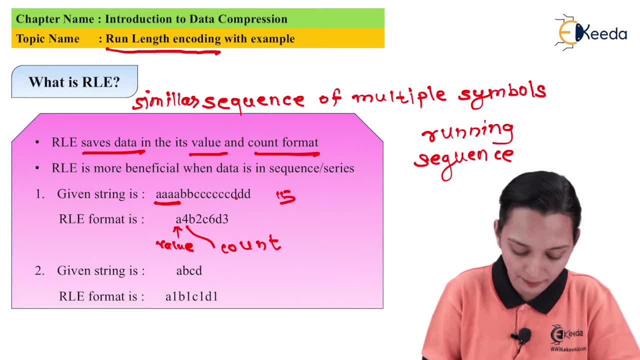 format. and finally is d, so d appears three times. so d is the value and three is the count. so if you are going to observe now this particular output, then how many bits or how many character it try to store, that means indirectly space. so that is one, two, three, four, five, six, seven. 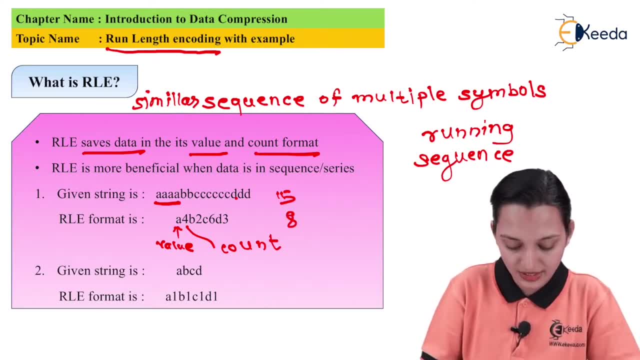 eight. So instead of using space 15, one, five, now we achieve the compressed size. try to understand, if I want to decode this data, then what I can do: a4, b2, c6 and d3. simply, I will write down the value first, a. how many times it appears: four. so one, two, three, four. after that, b. how? 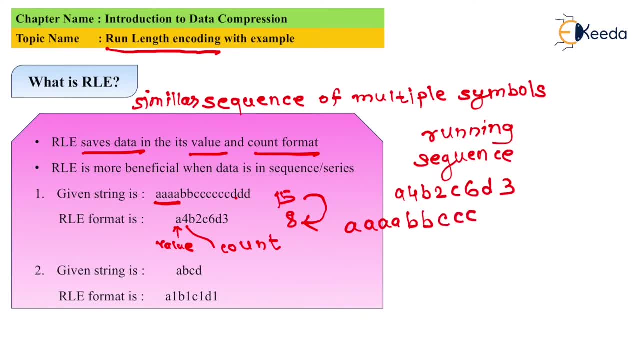 many times it appears two, one, two c123456 after the d. so, as it is, whatever the input present in the given string, that complete input I will get or I can achieve. as it is at the output side, that is nothing but what receiver side, and if I want to send this particular string, what I can send instead. 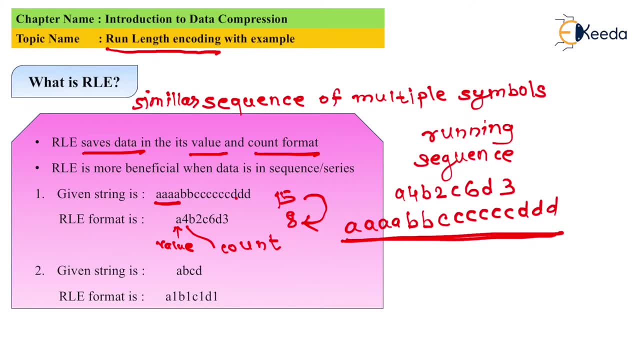 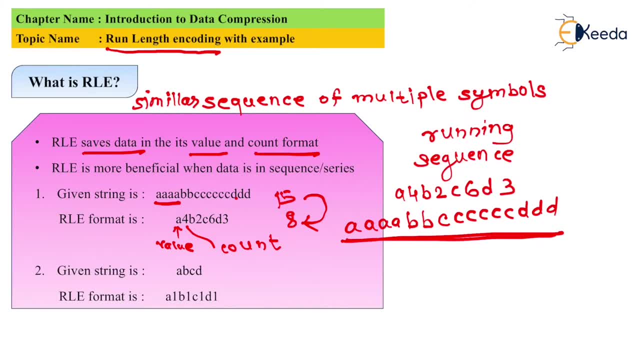 a4 c603. so here I try to compress the size of the data, but here I m not going to lose any value in the data. so this is known as the lossless data compression method. so you are getting success too, as it is forward or transmit a string at the receiver side using 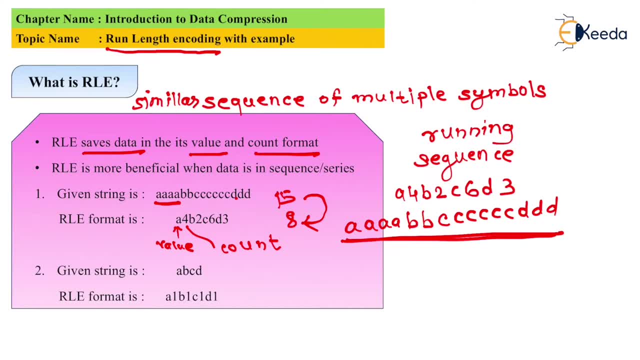 the data compression and why it become possible because of our lae. so within a minute we can go back encode the data as well as we can decode the data, so that it is very simple method of the data compression among all the methods. Now, I already told you, RLE means similar. 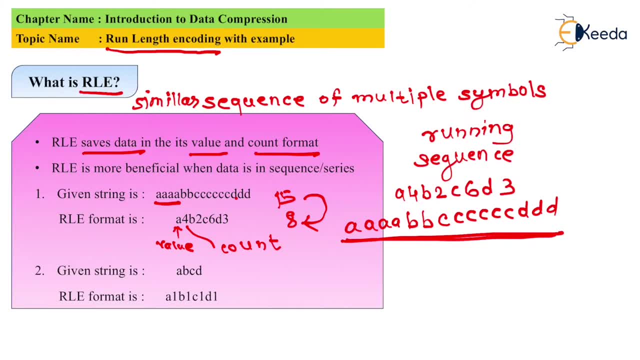 sequence of multiple symbols Here. if you are going to use only one symbol, then what will happen? Suppose I am going to write down the data like A, B, C, D- Again the multiple symbols first of all we will take- and it is RLE format- A. A is nothing but what Value, And one is what. 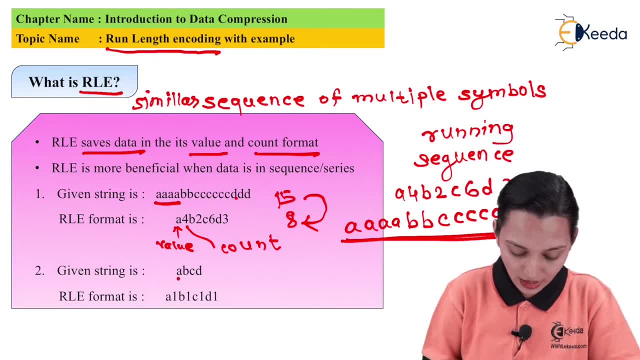 Count of that particular value in the string. So how many times A appears in the given string? Only one. So A one B, one, C appears only one time. D appears again, only one time. How much bits you required here to save the characters One, two, three, four, Four And? 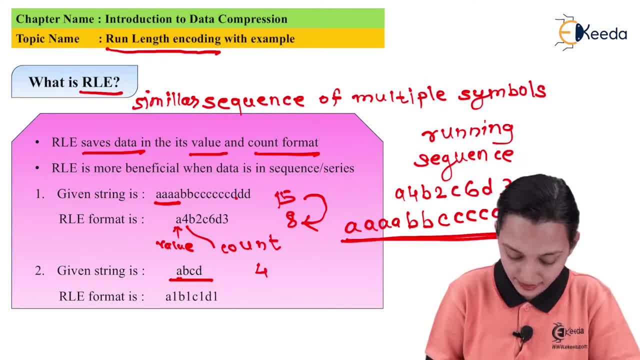 how much you required here: 1, 2, 3, 4, 5, 6, 7, 8. that means sometimes, in one case, are really is not more beneficial or it is worst in this particular case why? because if you are going to convert a given string, which 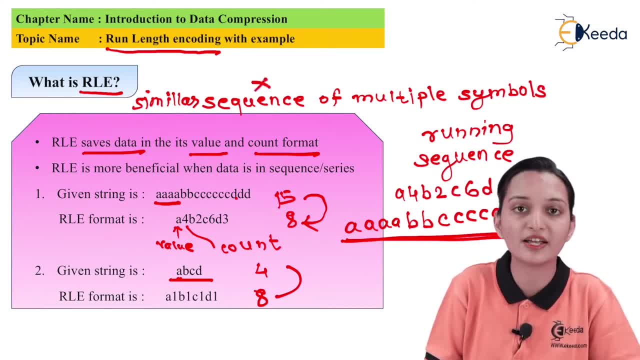 is not a sequence. if it is not a sequence of the symbol, then you may achieve the increment in the size instead of compression in the size. so in that particular case, where the sequence is not present, then that will be less beneficial. or you can say: this is the highest drawback of rle. so 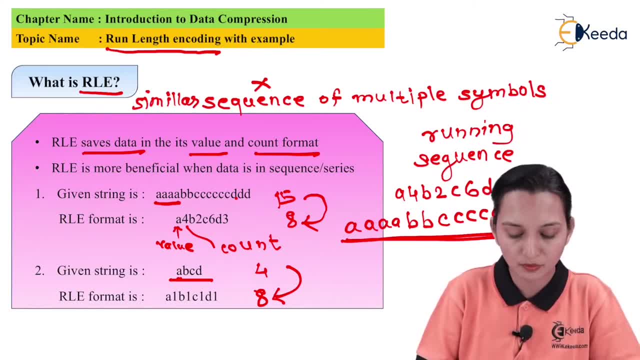 the next point is multiple symbols by multiple symbols, because whatever the number of data, if it is huge, then rle will be more beneficial. so, though the multiple symbols are not there, here we are can modify single or multiple, because if a appears thrice, then i can write down what a. 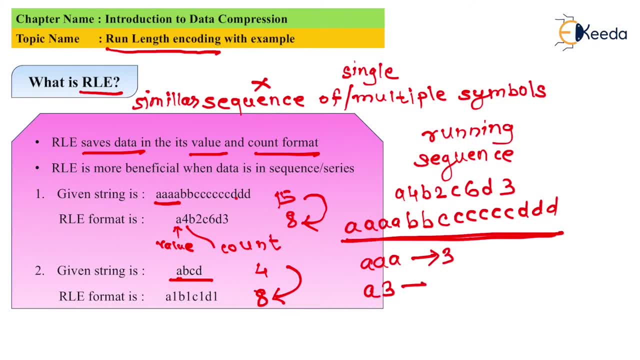 three. so here how much bit i required: three. here how much bits are required: two. so again, it is beneficial for me. so though the symbol is single or multiple, then also it is more beneficial, but most probably rle we used for the huge amount of string where it contains a number of data. 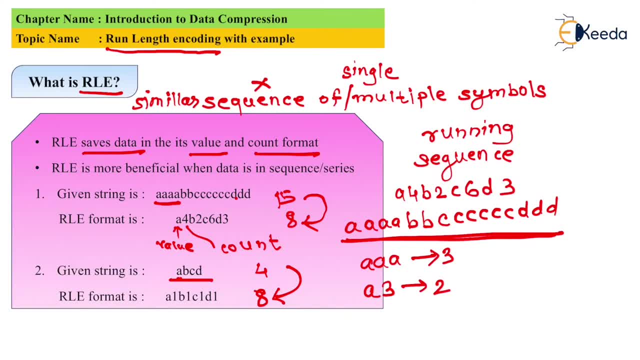 and this is the drawback of rle, where the sequence is not present. so it saves the data in its value and count format, no doubt, but it is more beneficial when the data is in sequence or series. this is the proof of our this particular statement. so, in this way, this is the first example which 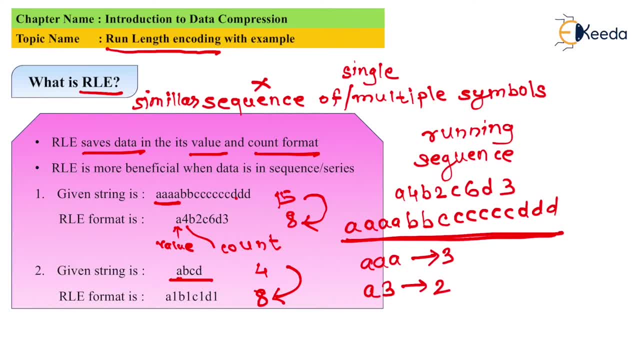 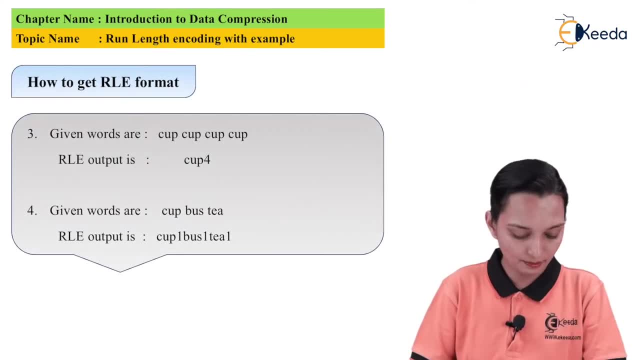 you can use to convert the characters into the rle format. so like that we will go for the second example. so the next example for rle is: given words are c? u p cup. i try to write down this particular word four times, so if you are going to observe this space also going to count when you will count. 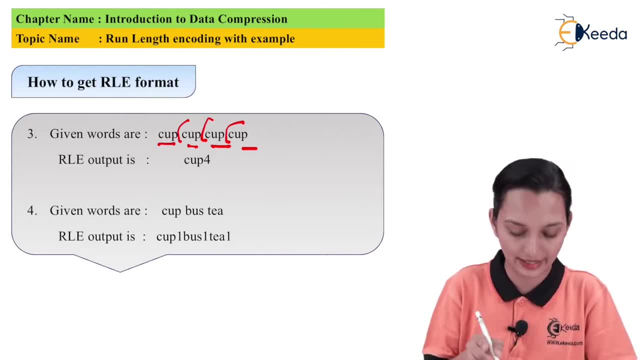 the size, so c u p and plus one size, so that is nothing but 3 into 4, 12, 13, 14, 15. again, it will take 15 size to store this particular words and rle format is c? u p and how many times the data is. 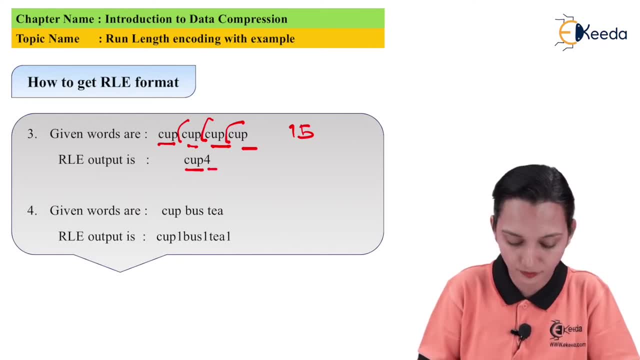 what c, u, b, how many times count is nothing. but what four it appears in the string four. so that will take only four sides to send the data, to store the data. so again you are able to achieve the good compression while transmitting the data. but similarly, when the 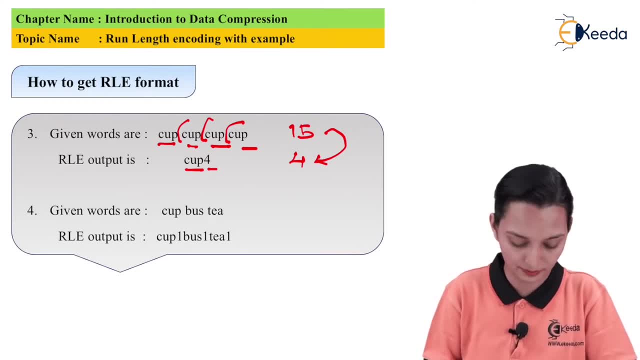 words are different or appears only one times. then cup, it appears one time. again the space after the words bus, it appears one time, and t, it appears one time. so it's rle format. here you are able to write down this particular given string in the three into three nine. 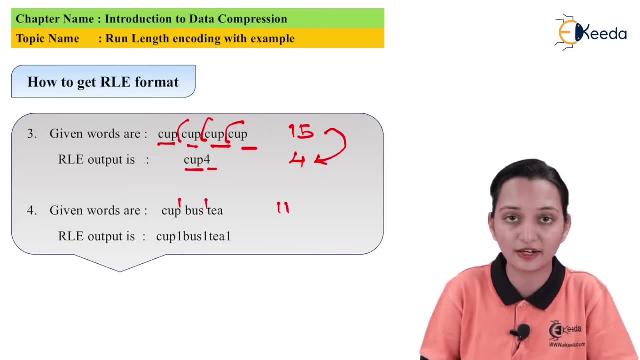 in eleven. so eleven size will require to store this string. and rle output is what c u p cup. it appears once. b u s bus. it appears once. t a t. it appears once. that means what three, three, three and one, two, three, twelve. so size is going to increase after the rle output when the sequence 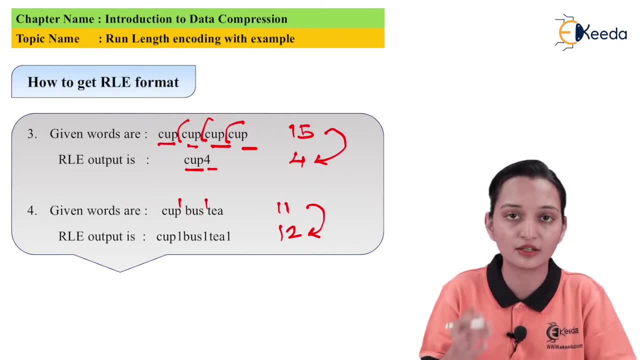 is not present. no doubt here multiple symbols are present, then also it is okay. but if the sequence is present, then rle is able to compress the data size and so that sequence is important in terms of characters, which we have seen in the previous example, in terms of words also. 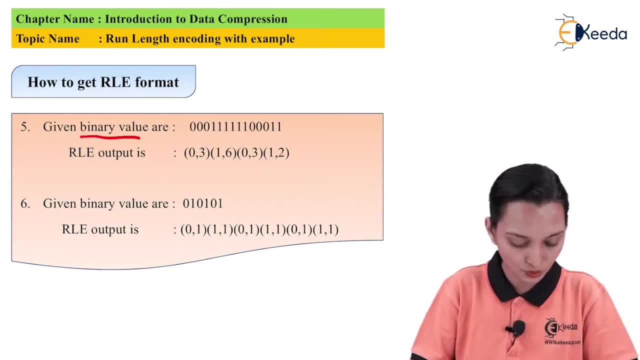 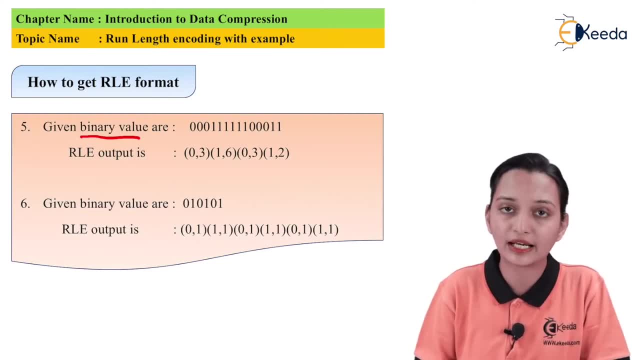 zero, zero, zero, one, one one. this is the string of the binary number. if you are able to convert the, the given string, How we can write down into the RLE format: 0,. it appears This is the data value 0. But as the format is binary, how to represent it In a bracket comma? How many times that? 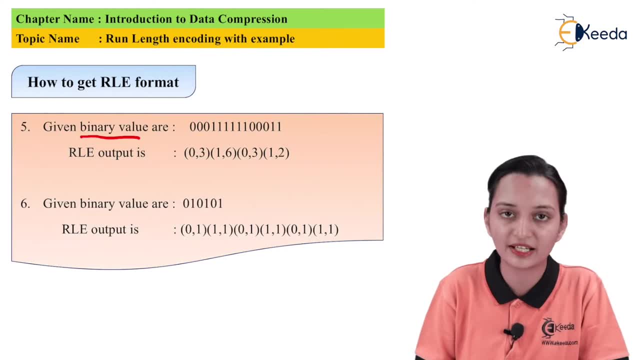 appears 3 times Again: 1. How many times that appears? 6 times. Separate it with the help of comma, Then 0,, 3 and 1, 2.. So it is very easy to transmit this particular data instead of. 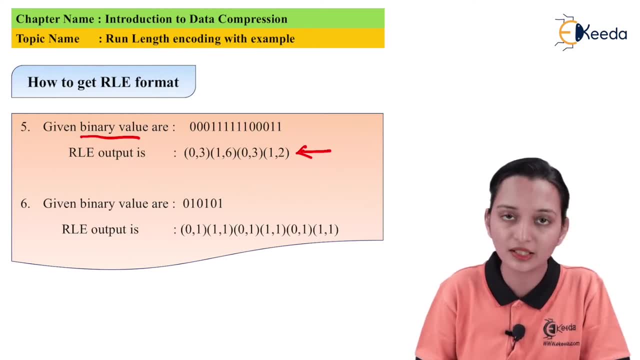 transmitting a huge string, Because while transmitting this data, the manual errors will be minimizes, While there is a chances of the manual error while writing down this data again and again. So this will be more useful as it is in the compressed form, But the binary value. 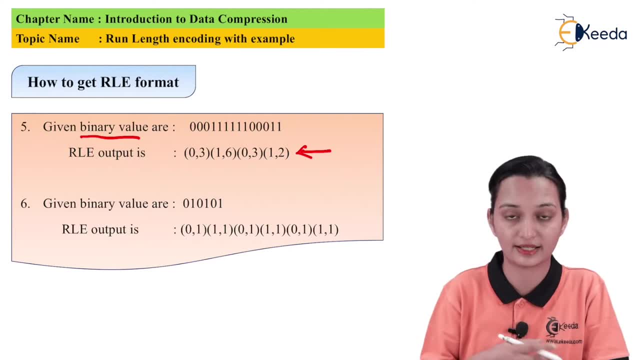 when the given binary values are not in the sequence, then what will happen? 0, 1, 0, 1, 0, 1, 0.. In the sequence of the string. again, you cannot calculate the 0 where, if you are going to calculate like, 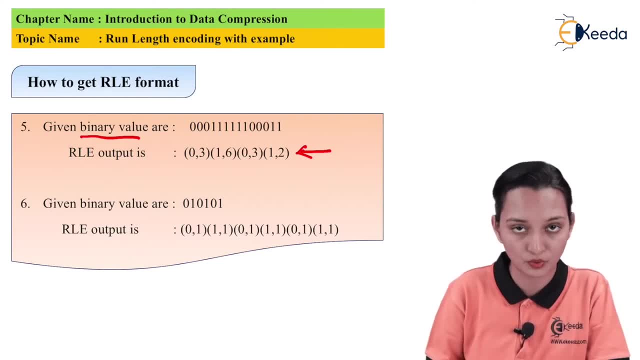 this 0, it appears 1,, 2,, 3.. No, it is not good. You have to calculate the sequence of the data in the series itself. So 0.. 0 appears once After that where the 0 appears, Yes, but not in series. 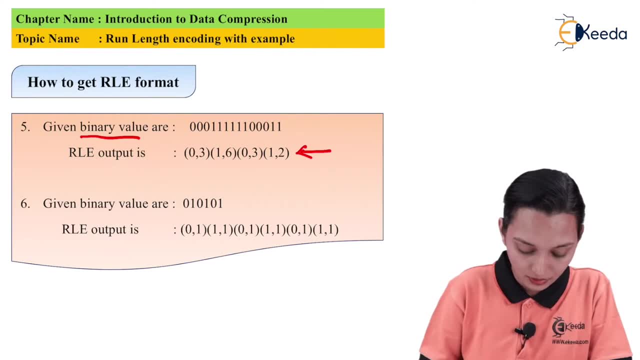 So draw another column, So 1.. 1 appears. how much time? Only once Again after this 1, where 1 appears? Yes, it appears, But there is a 0 present in between these two 1. So 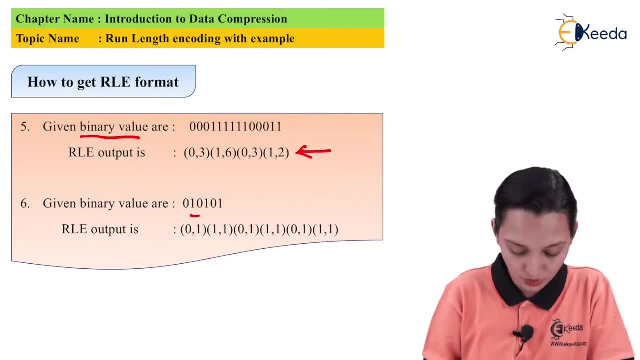 you must have to again draw a bracket for this 0. So 0. It appears how much time 1.. Again, 1 appears how much time 1.. So if you are going to observe this obviously here, the size required to: 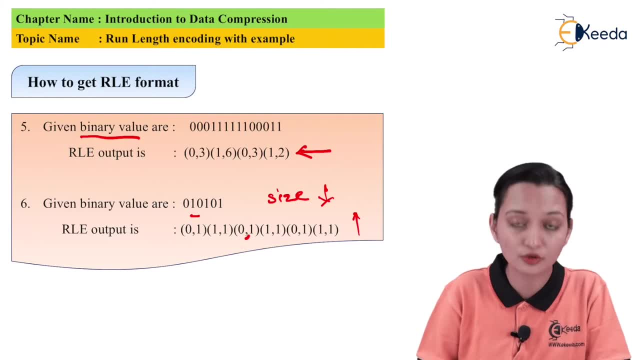 say 0 is 0. So if you are going to observe this, obviously here the size required to say 0 is 0. So store the data is less, But here the size required to store the data is high. That means 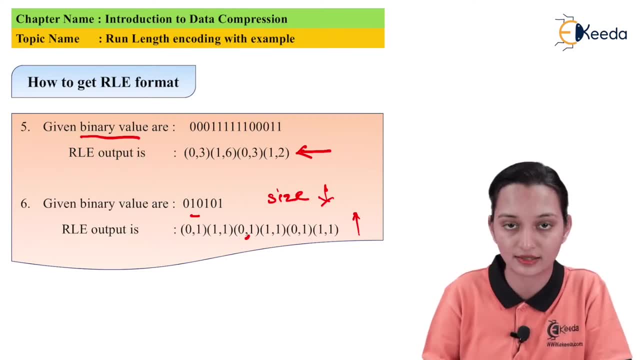 when the binary values are also not in sequence, then RLA is not useful. So always, whatever format you are going to take, that should be in the given sequence. Otherwise it will be the worst case to transmit a data by transmitting your given format into RLA. So this is the best. 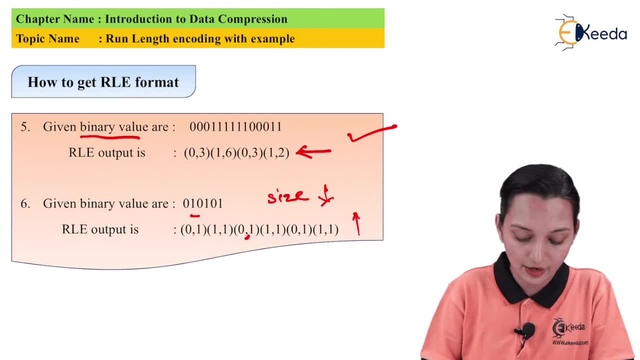 example of the binary value. Similarly, I have already told you: if you are going to use this bus bus, then the RLA format will be bus 2.. So how to decode this format? Write down the value, How much time it appears, Write down it. So this is nothing but decoding. So, after encoding the 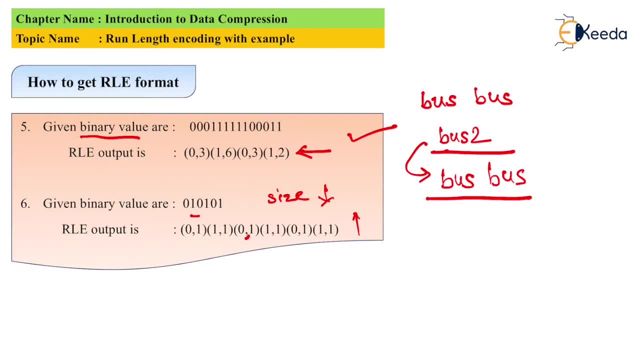 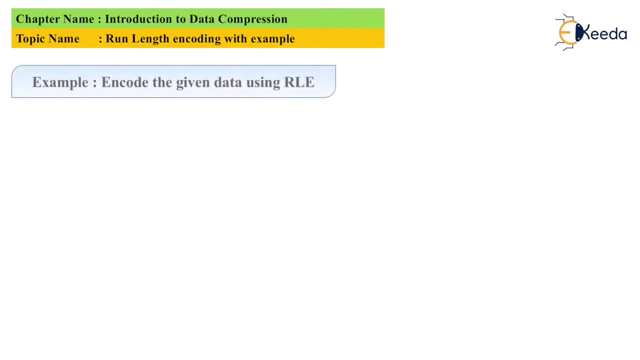 data. you are getting this, But what will happen while decoding the binary values? That kind of questions are always asked in your example, So we will try to take that particular example to solve for RLA encoding. So this is nothing but the example. The given words are: 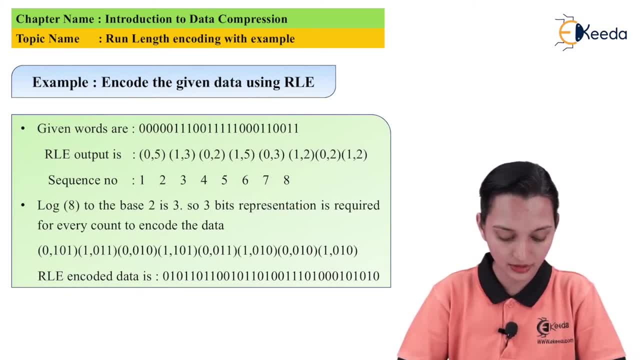 0000011100111111000110011.. This is a huge number of string. That means the number of data in string, But whenever we are going to convert it into RLA, that will look more simple. So try to convert it. 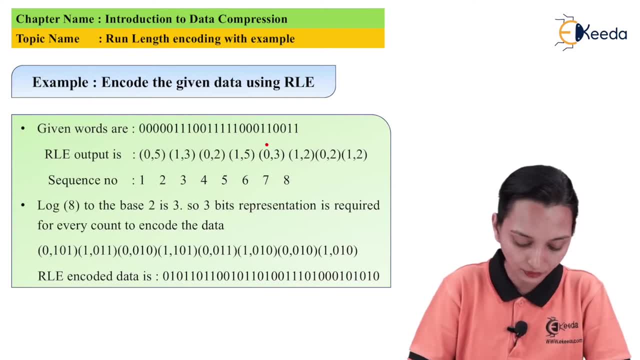 into RLA output. So RLA format is what Value and count. So what is the value? Value is 0.. First 0 appears. How much times it appears? 5 times. So 0, 5.. After that 1 appears. 1 appears 3 times. 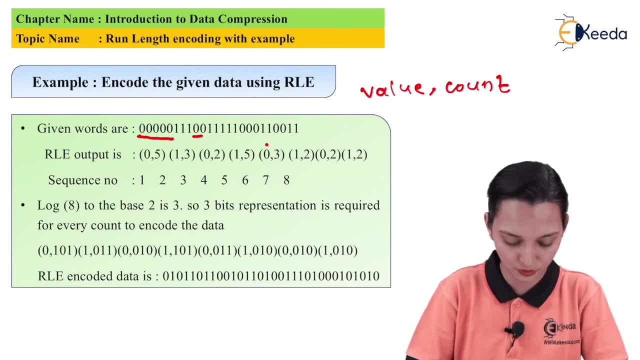 0 appears 2 times Again, 1 appears 5 times, 0 appears 3 times Again, 1 appears 2 times, 0 appears 2 times, And last one is again: 1 appears 2 times. So this is nothing but RLA output. So 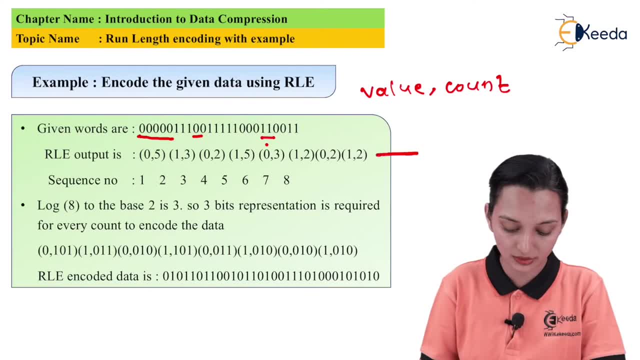 now we have to go and decode the data. That means by using this particular input. we required a string or the words. So let's say: given numbers are, So now you have to give the sequence. Sequence for this, every bracket, So like that this is nothing but number 8.. So 8 brackets we have used to write. 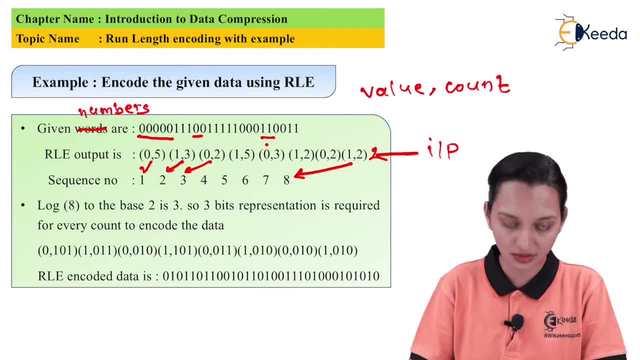 down the combination in terms of value and count in the RLA format. So the highest value of the sequence number is what It is, 0. So let's go and decode that. So now you have to give the 8.. Now the next tip is log of this highest value to the base 2.. Find out that answer Now. here you. 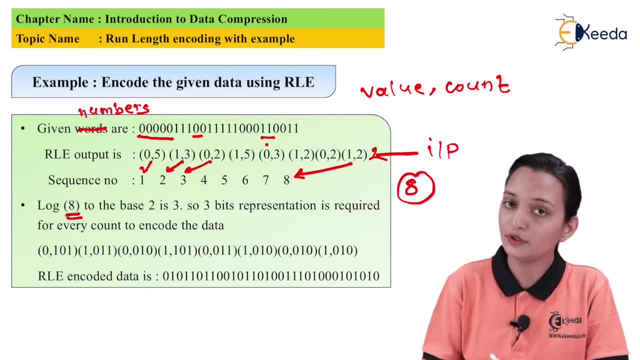 are getting the highest value, 8.. So log of 8.. If not 8, in other examples you may or may not get 8.. So what is the equation or what is the formula: Log of the highest value which you are getting with the help of this count of the sequence That you have to write down and find out the answer. 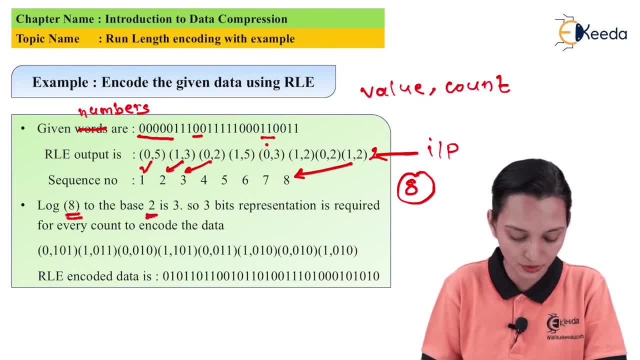 for that particular highest value to the base 2.. So now I am getting here highest sequence 8.. So log of 8 to the base 2 is nothing but convert it into log base 2- 10. Why? Because our calculator is familiar with log 10.. So log 8 divided by log 2. This is nothing but base. 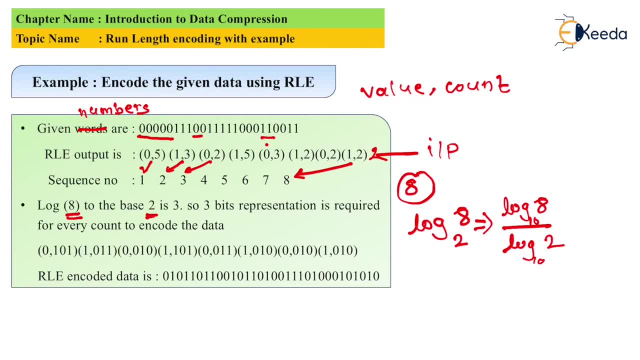 10 answer. So simply you can put up in your calcine log 8 by log 2 and you will get the answer 3.. So now it means 3-bit representation is required to write down this count, Not a value to write down the count. So count you can encode with the help of this 3-bit. 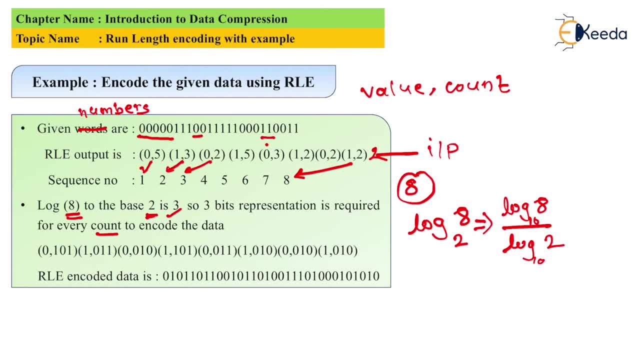 representation. And already the values are in the binary format. Why? Because the given numbers are in binary format. So here also the values. every value is already in binary format, But count is not in binary format. So it is our duty to convert the count in binary format. But how? With the help of how? 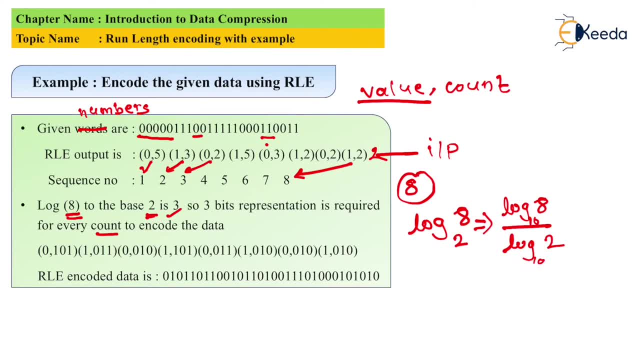 much bit that we have to find and that we can achieve with the help of the highest sequence number. Take the highest sequence number, log to the base 2. Find out the answer for the count value, And that answer will be the representation of the bits which we required to convert it into. 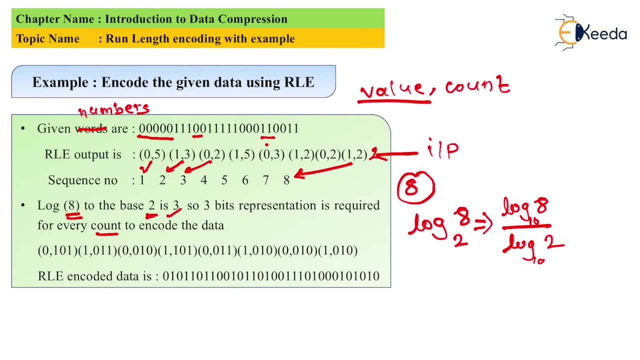 the binary. So now we will try to do it. So for the first column that is nothing but what? 0 comma 5.. So 0 write down as it is. After that, 5 convert into the 3-bit representation of the binary. So what will? 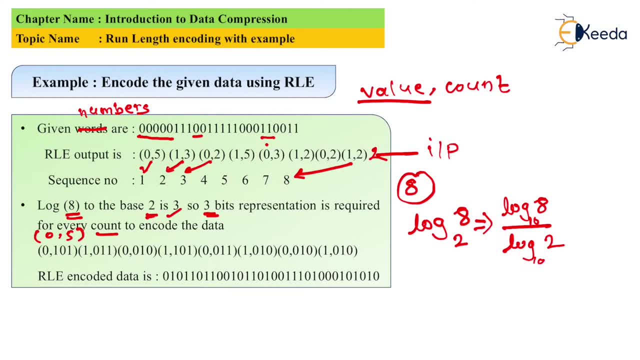 be the value 1, 0, 1.. After that, 1 comma, 3. This is nothing but what 1 comma 3.. So 1 as it is comma 3.. 3 is conversion in binary: 0, 1, 1.. After that 0 comma, 2.. So 0 comma. 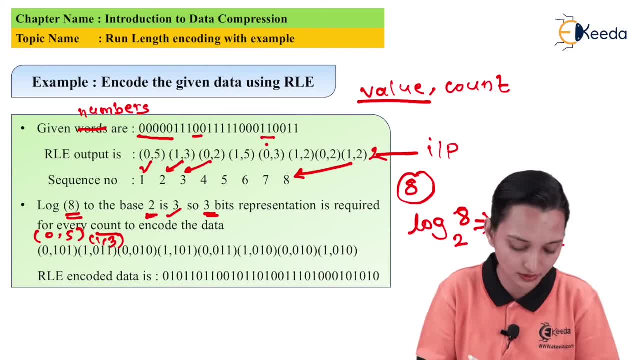 Now what is the binary conversion of 2 into the 3-bit? That is 0 1 0.. After that: 1 comma: 5.. 1 comma: 1 0, 1.. Similarly for 0 comma: 3. 0 comma: 0, 1, 1.. For 1 comma: 2.. 1 comma: 0: 1, 0.. For 0 comma: 2. 0 comma. 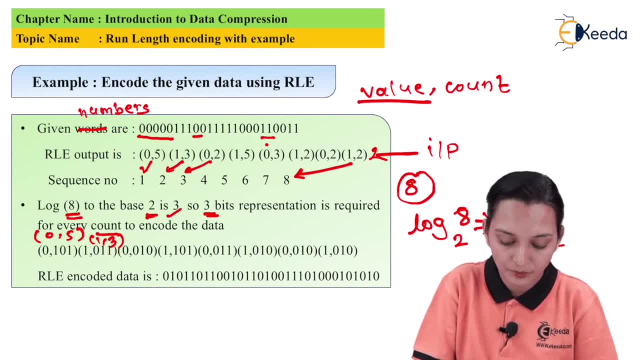 0, 1 0.. And finally, for 1 comma 2.. This is nothing but what Value and its count. So 1 comma 0, 1 0.. Now the conversion of count into the binary. Already the value is in the binary form, and now 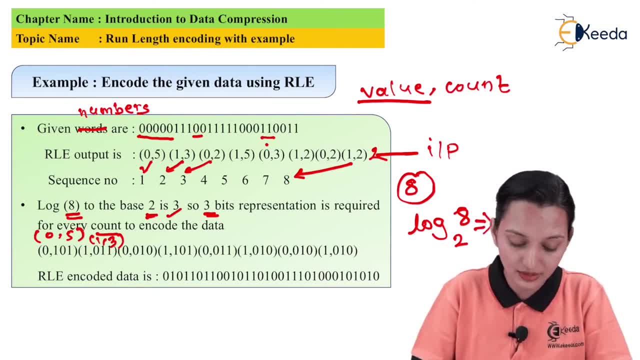 you are getting success to convert. the given count is in binary form. So the final answer after RLE encoded data is what? Remove this comma, Remove the bracket and write down this value. So this is nothing, but what The final answer after encoding? 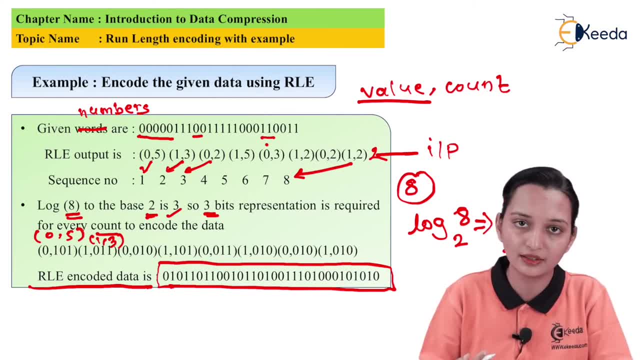 So this is the encoded data. Again you are able to decode it and again you are able to achieve the given string. So in this way you are able to do the RLE encoding. This is nothing but the encoding, Not decoding. After decoding the data, again you will get what The previous string as 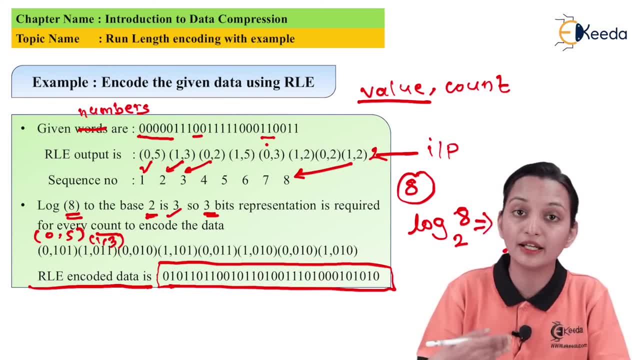 it is So RLE output and RLE encoded output. These are two completely different things. So RLE output means Just format representation And RLE encoded data means, again, you require to convert that format into the given example format. As the given example is in binary format, you have to again. 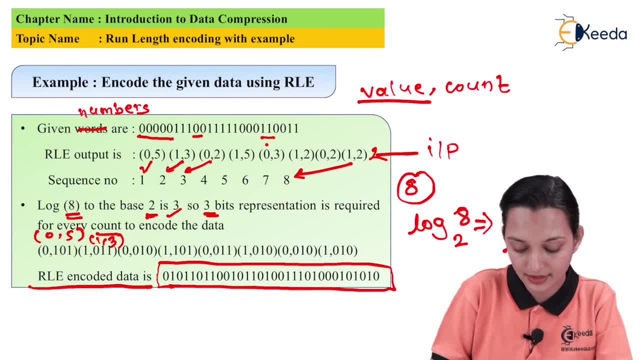 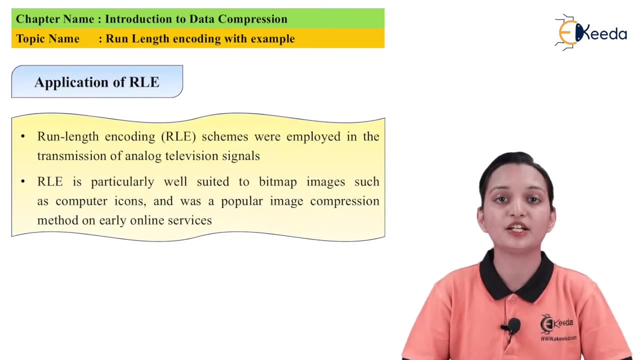 encode this complete data into the binary format And this is nothing but what Encoded output. So RLE encoding part is always frequently asked in your exam and this is the generated output. with the help of that, Now, the applications of RLE, Where the RLE we can use. So such kind of example in terms of 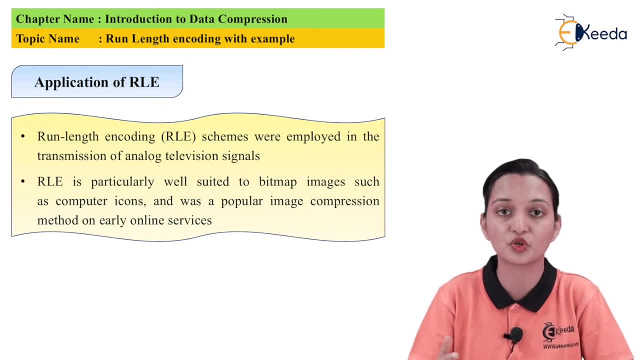 binary in terms of words, in terms of characters, in terms of symbol. we have seen how to convert that into the RLE and it is more beneficial, no doubt, But where exactly that particular encoded or decoded output is going to use. The first one is: these were employed in the transmission of 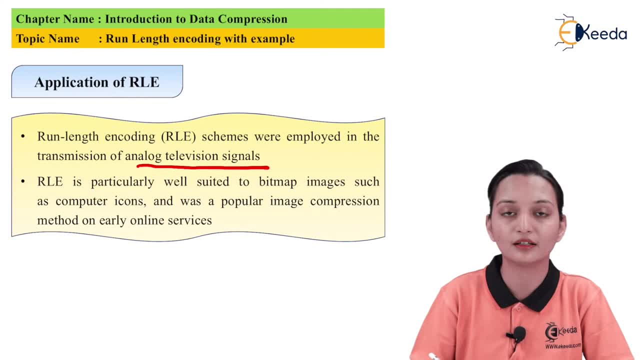 analog television signals. We all know that the RLE encoded output is going to use the analog television signals. We all know that our signals and their values are continuous and in the sequence series of sequence. So, while writing down the one exact value, along with the count for a particular signal or the